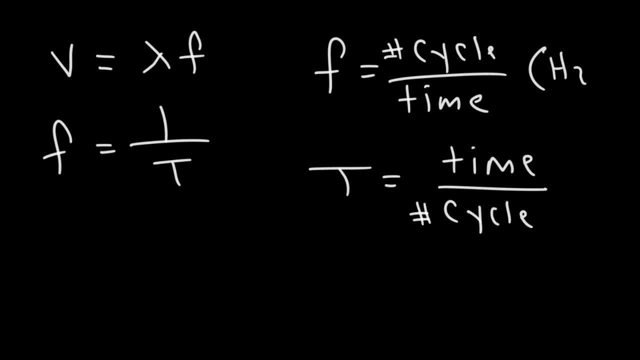 The frequency can be measured in Hertz or one over seconds. The period is typically measured in seconds. So those are some equations that you may need to know when dealing with waves. Now let's talk about transverse waves. What do you think a transverse wave is? 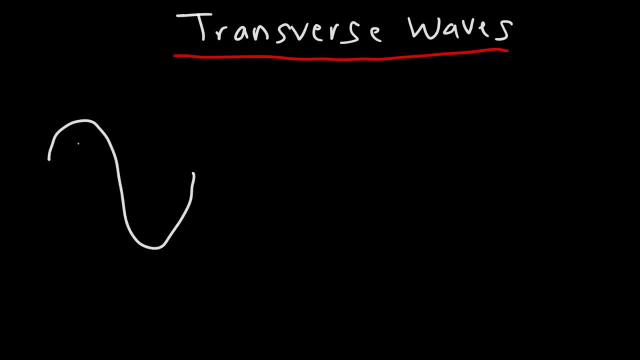 The wave that we drew earlier is an example of a transverse wave. The reason why it's a transverse wave is because the wave is moving in the x-direction, but the oscillations are in the y-direction Anytime the oscillations are perpendicular to the direction of the wave motion. we're dealing with a. 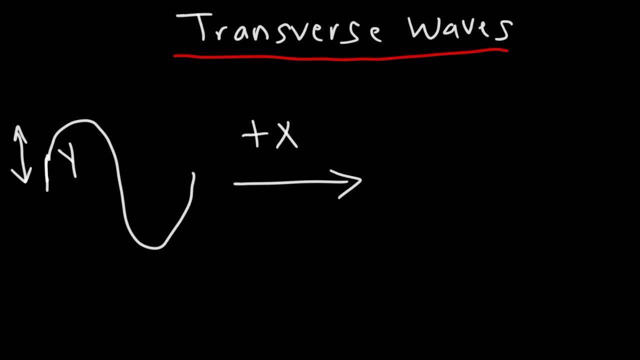 transverse wave. Examples of transverse waves include water waves. let's say, if you're on a beach and you see those waves on the ocean, those are transverse waves. EM waves are also transverse. so these are electromagnetic waves such as light waves, radio waves, infrared rays, x-rays, gamma rays, ultraviolet. 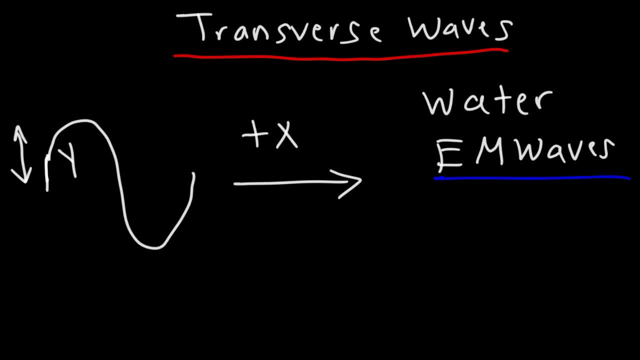 rays from the Sun. All of these are transverse waves. Another example is if you have a string and if you pluck the string, that's going to create a transverse wave. It's going to oscillate up and down while appearing to move left. 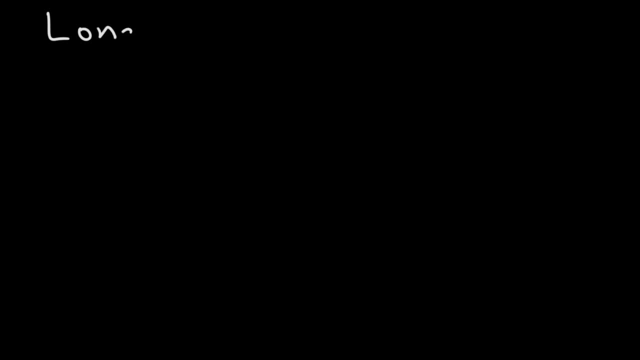 and right. The next type of wave that you need to be familiar with are longitudinal waves. Now, longitudinal waves are different than transverse waves. In transverse waves, we said that the oscillations and the direction of the wave motion, they're perpendicular to each other. Well, for longitudinal waves, 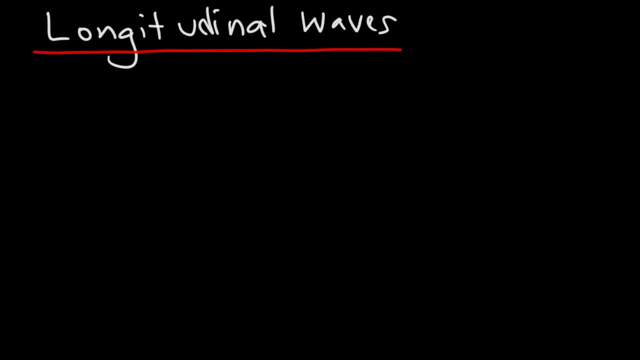 the oscillations are parallel to the direction of the wave motion, So let me see if I can draw a visual illustration. So notice, here we have a region of compression and here the wave is expanded, sometimes known as a rarefaction. So the wave is moving in the